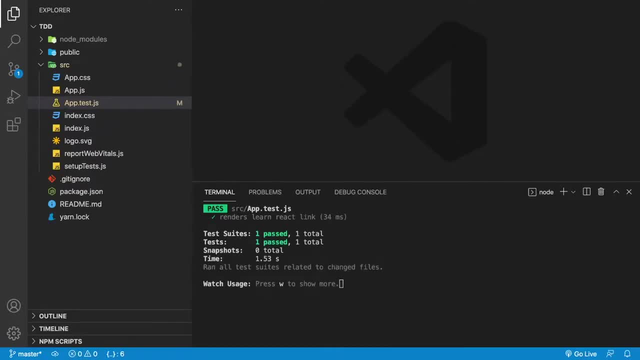 going to hit enter to just watch all of the files. The default React application comes with one test and we can see that one test is passing. To ease into the TDD workflow, we're going to start by writing one test and then we'll make a list of tests for our awesome counter. Let's start with. 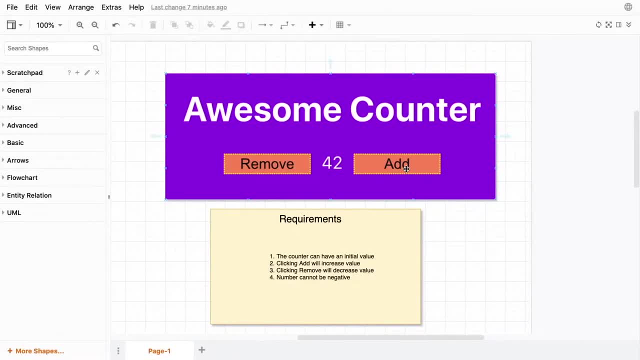 the very first test that we need. Looking at our application, one of the most notable things is that we have a title called awesome counter. When our application starts up, we want that title to be there, So let's go ahead and write that test. We'll start by going to app testjs and inside. 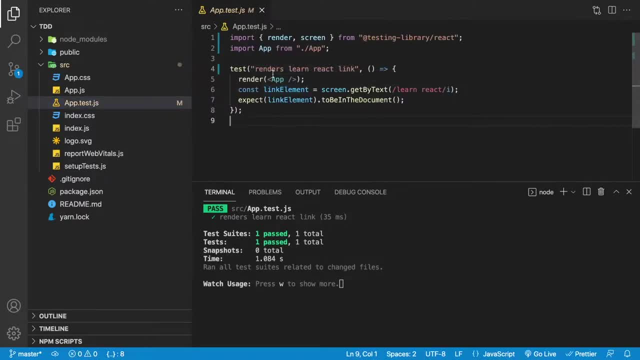 app testjs. what we're going to do is we're going to repurpose this test over here because we're not going to have this text anymore on the screen, So we'll go ahead and rename this over here to. it should have the correct title And the title that we're going to be looking for. 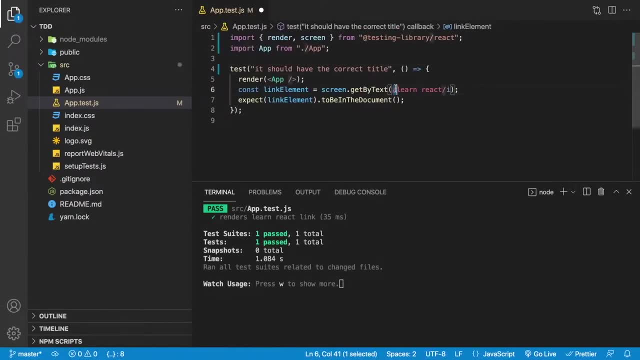 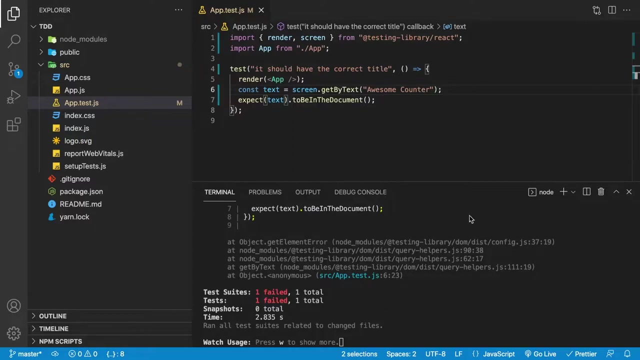 is awesome counter, So let's modify the text over here And we're going to modify it to awesome counter. You spell that right. then we're going to rename link element to text. As you can see, we now have a failing test. This is the test driven development workflow. we've written a. 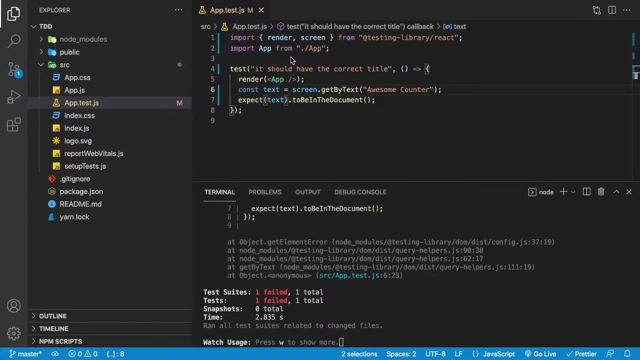 test, it's now failing. Now we're going to go write the code in order to make it pass. It's up to you to go ahead and write good code to satisfy your tests. Your tests will typically drive you in a path that makes you write good code. But what I could? 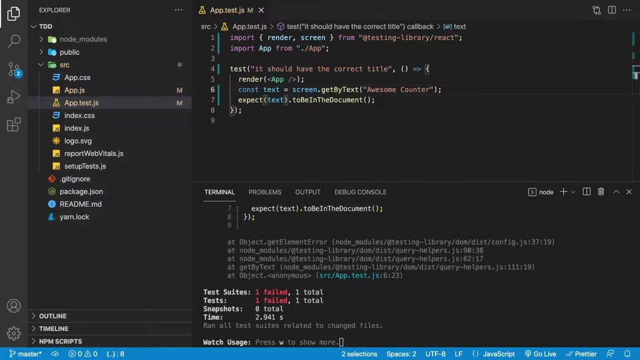 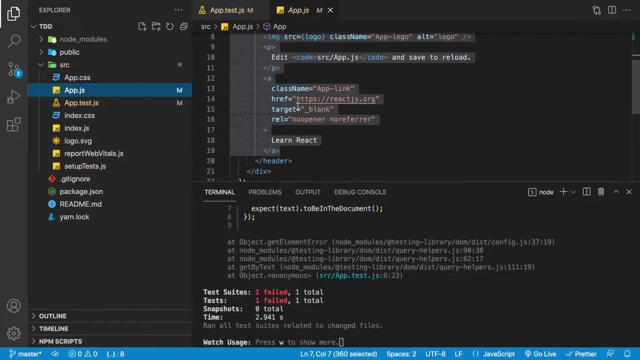 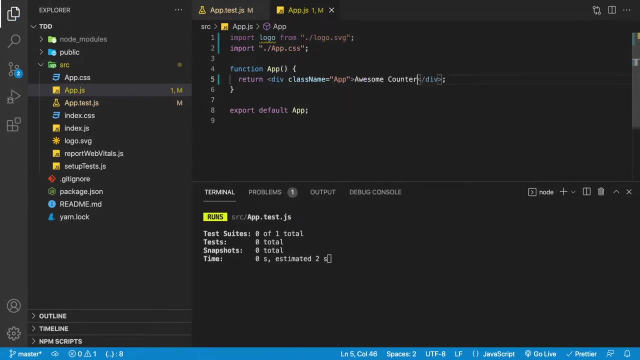 do for this particular test, because it's so generic and we're just looking for some text on the screen- is I could go to my appjs, delete the contents of what we have inside our appjs and just kind of leave that div there, And if I put awesome counter here and save it, our test will be passing. 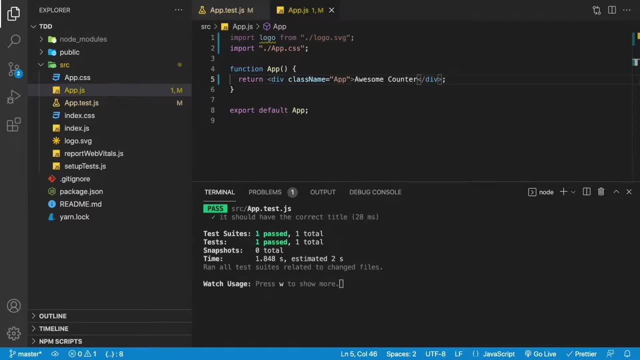 you typically won't want to do this because you want to write the best code. However, I just want to show you that you can make it pass. So let's go ahead and write the code And we're going to make your test pass in different ways. I've actually done this before in something called. 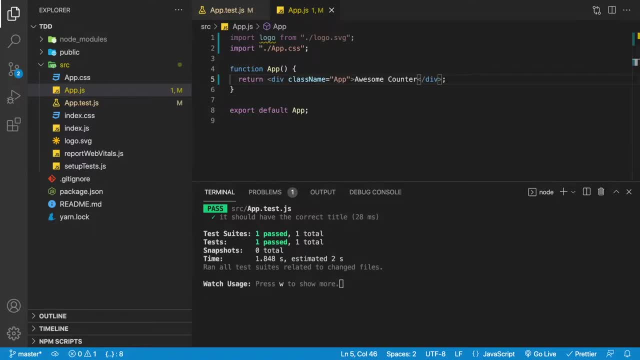 pair programming, where you work with another person, And we did this little process of ping ponging where one person would write the test and the other person would make the test pass, So you could come up with all kinds of weird ways to make the test pass without actually. 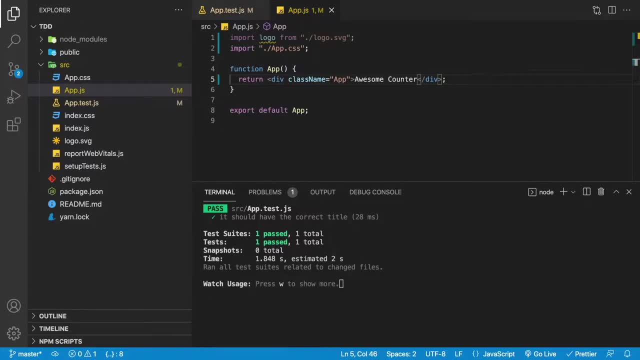 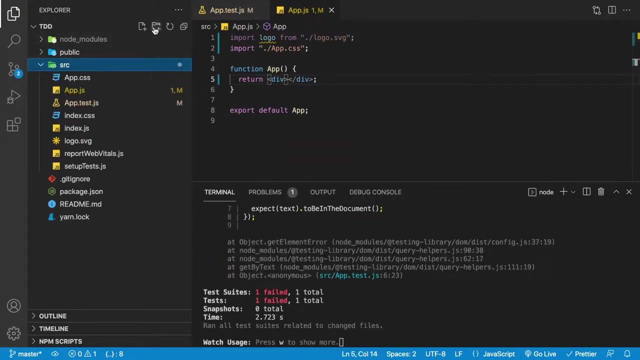 satisfying it, which then forced the test writer to write better and better tests, which would force you in the direction of writing the best code. That being said, we're going to go ahead and delete the text over here that says awesome counter. We'll just make this an empty div for now. then we're going to go ahead and create a folder over. 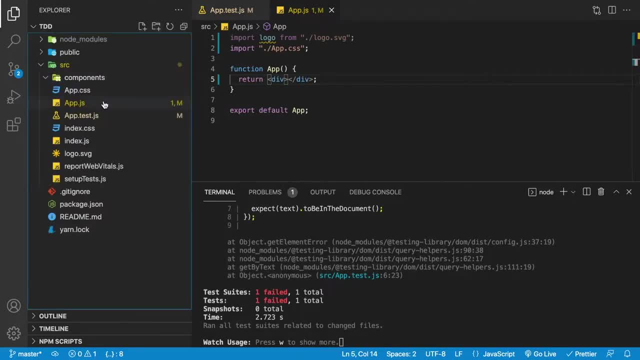 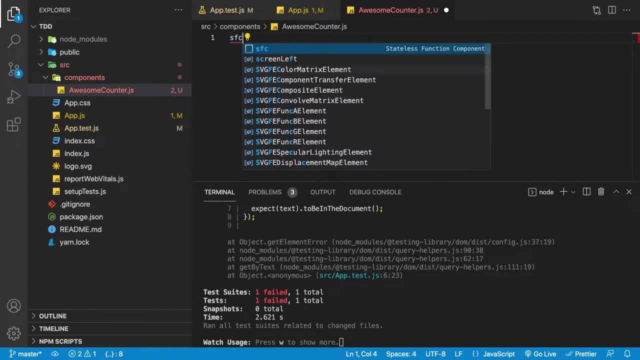 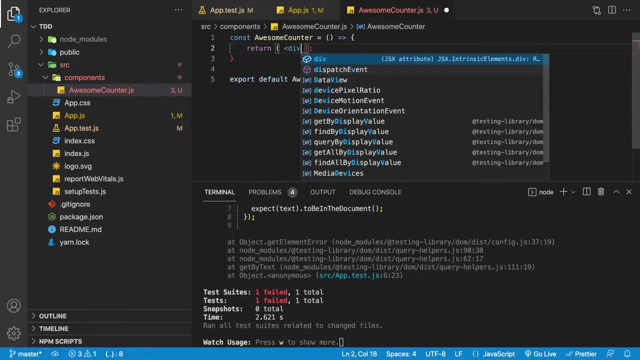 here And we're going to add a new component. we'll create a component called awesome counter JS, And then inside here we'll just declare that component And I'm just using some shortcuts over here to quickly create it. we have our awesome counter And in our inside, our awesome counter. 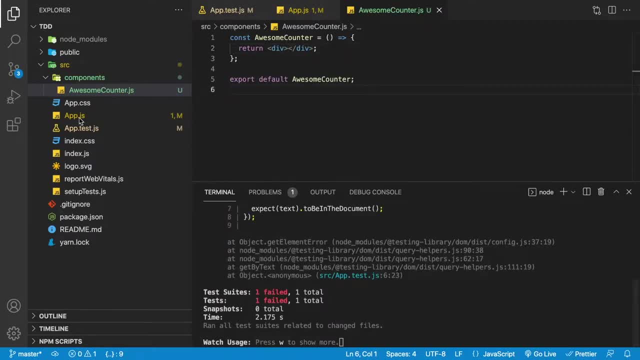 let's go ahead and just save that with the empty div. We'll then go back to our appjs, where we'll import our awesome counter And then use it. go down inside the div over here, we'll use our awesome counter And when we save it, 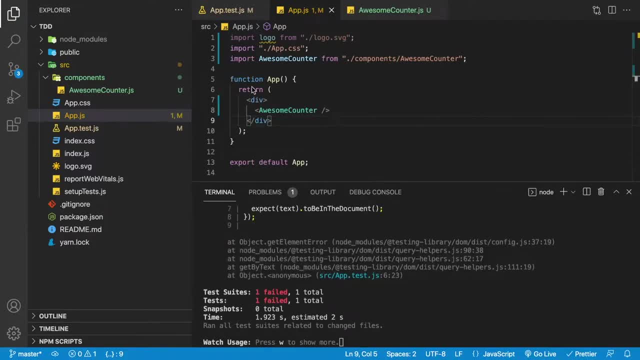 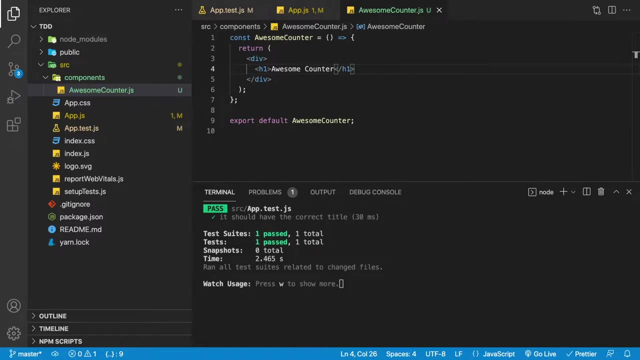 we're still going to be failing because it can't find that text. So then let's go to our awesome counter over here And we're just going to add an h1 inside that div And we're going to put our title: awesome counter. Now our test will be passing. pretty simple workflow. write a test. 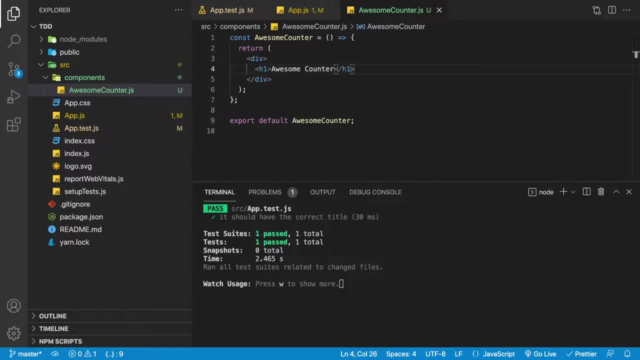 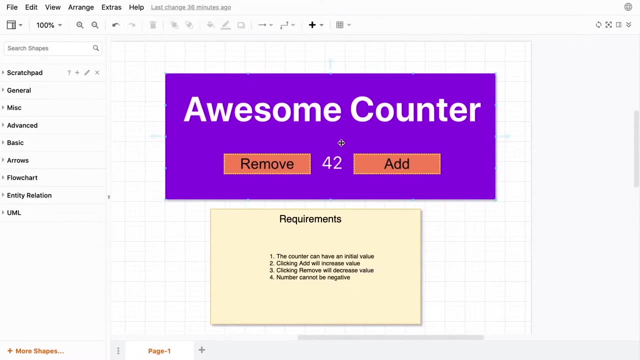 see it fail and then make that test pass by writing the code. Now let's up our test driven development game by looking at the remaining part of the application and what we need to write. the rest of the code that we're going to be writing is going to be inside the awesome 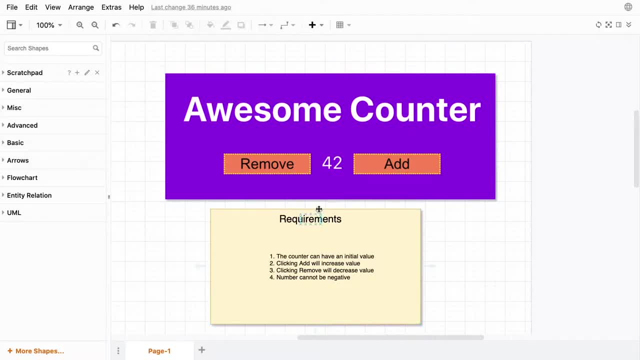 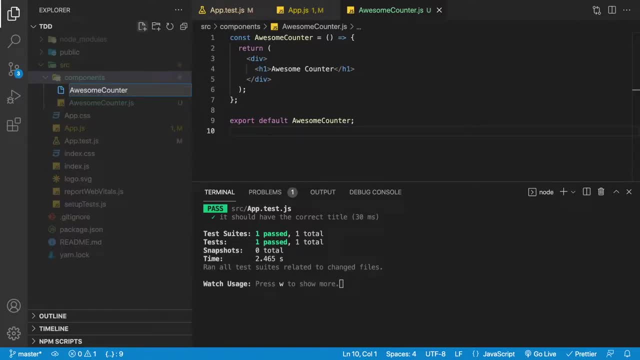 counter component. What we're going to do is we're going to come up with a list of tests. the way we're going to do this is we're going to create a new file over here for our awesome counter- And it's gonna be awesome- counter dot, test, dot, j, s- And we're going to write a list of tests, all of. 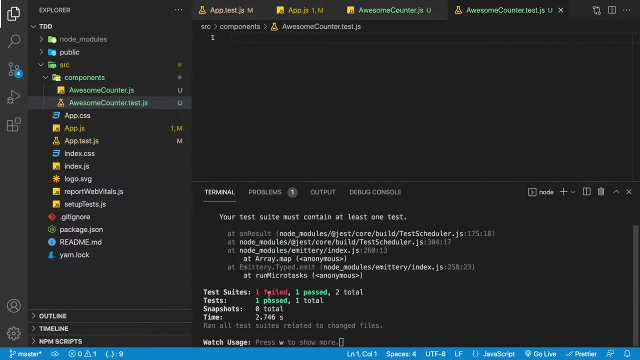 these tests will, by default, start failing immediately. we're getting a failure right now inside this file that we've created was a good start. let's start by writing that list of tests. So what we're going to do is we're gonna look at our awesome counter over here. look at the. 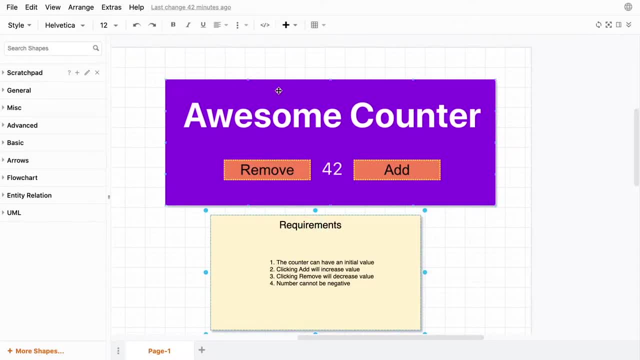 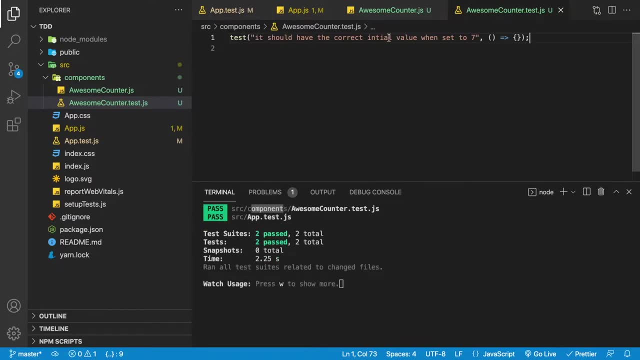 requirements. one of the requirements is that the counter can have an initial value, So let's go write a test for that. Here's a test that I've stubbed out. it says it should have the correct initial value when it's set to seven. However, we have a little problem here. the test is passing. 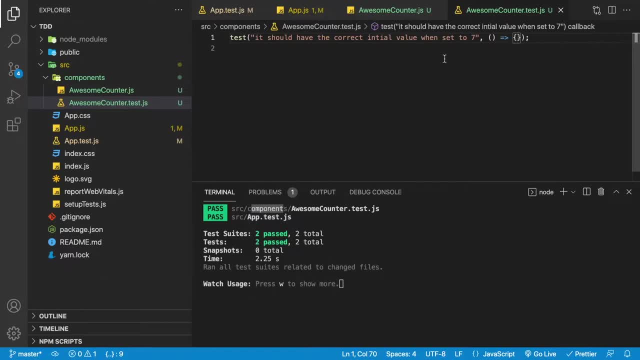 we don't want the test to pass. we're just stubbing them out right now. we're not going to write the full test, we're just going to stub them out In order to help this test fail. one thing to understand is the way a test framework works is when an exception is thrown, that means the test. 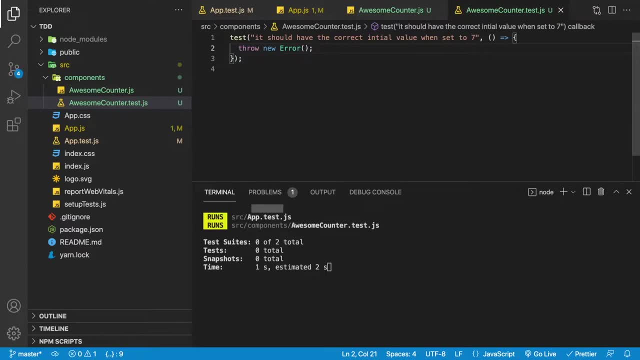 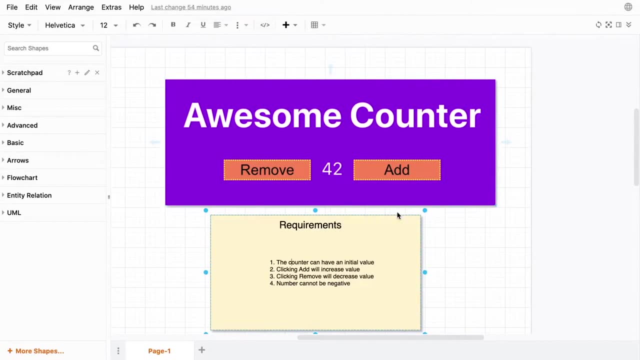 will fail. So if we do throw new error, the test will automatically then fail. And now we're getting that one failure. Let's go ahead and get our next test. Looking at our requirements document over here, we know that the counter can have an initial value. Well, what if we don't provide an initial? 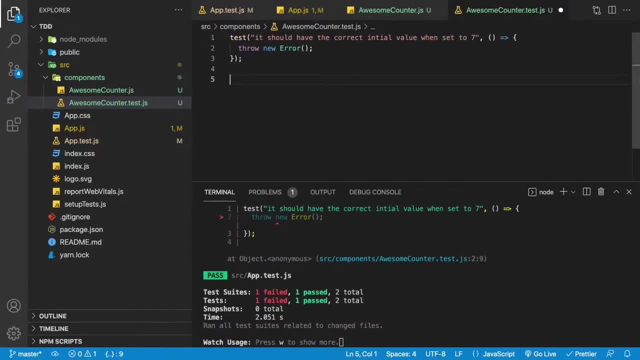 value. In our application, we're going to assume that if you don't provide an initial value, that the initial value is zero. we're going to add a test in order to reflect that. Now you can see that a requirements document doesn't mention a specific use case, And this is perfectly fine. 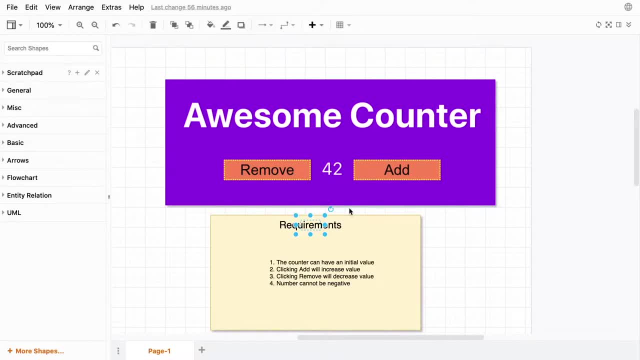 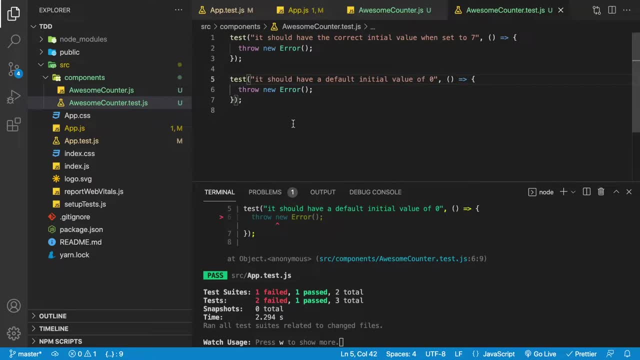 requirements document can't have every use case, But what's great about our tests is that our tests document how our application will work. The test will always be up to date and reflecting exactly what the code is doing. The requirements document is a lot harder to keep up to date than the tests in your application. 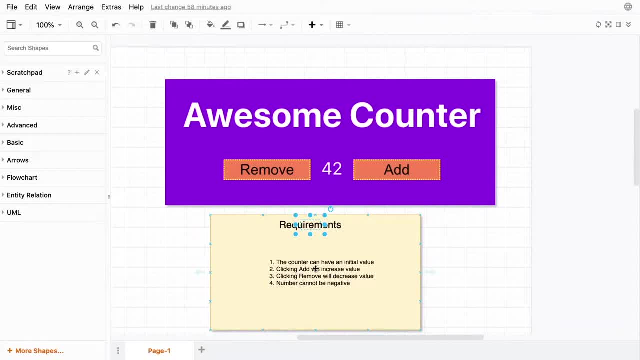 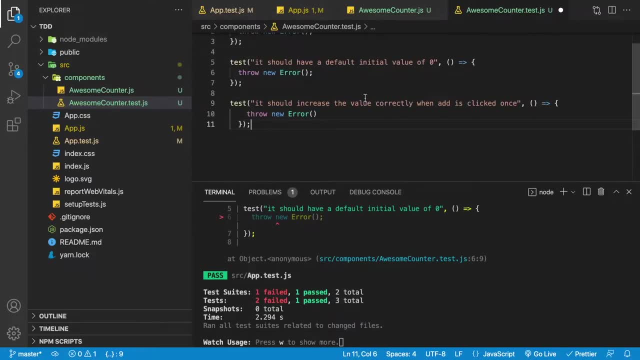 The next item from our requirements document is that clicking add will increase the value. Let's go ahead and add that test. It should increase the value correctly when add is clicked once. Well, if we have the use case for when it's clicked once, why not when it's clicked twice? 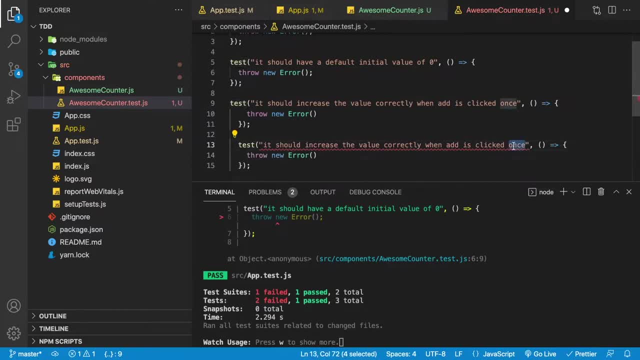 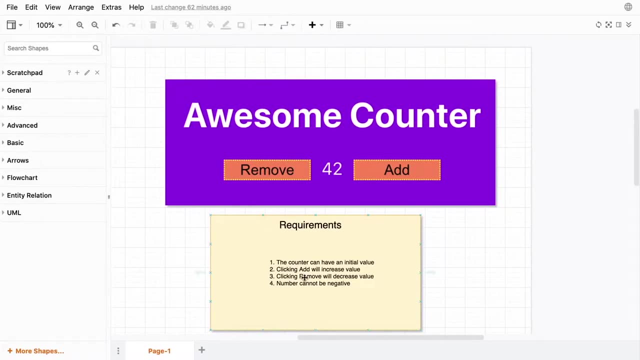 Let's go ahead and add a test for that. I'm just going to copy that one and change that one to clicked twice. Save that And now we should have four failing tests. We'll then go ahead and add identical tests for remove. So when it's clicked once and when it's 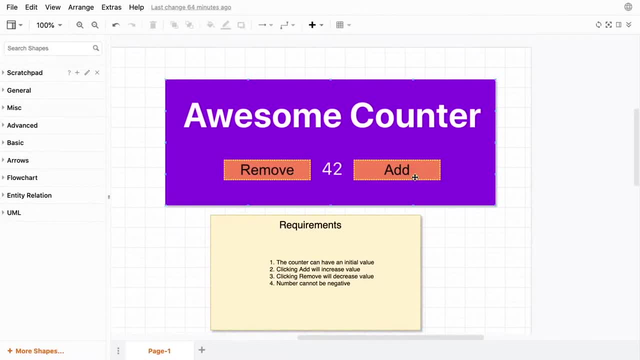 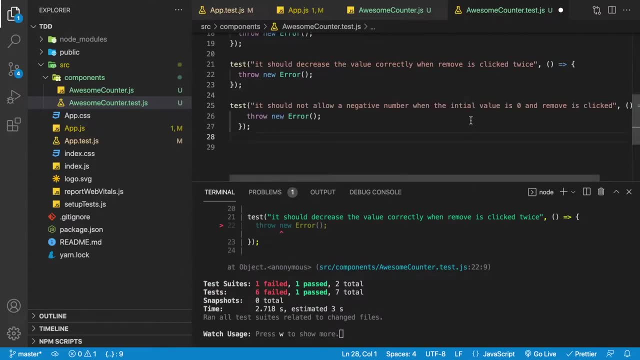 clicked twice and then we'll have six failing tests. The last requirement in our list is the number cannot be negative, So we'll go ahead and we'll add a test for that. Now this test is a bit more verbose, but I wanted to get the point across that did not allow a negative number when the 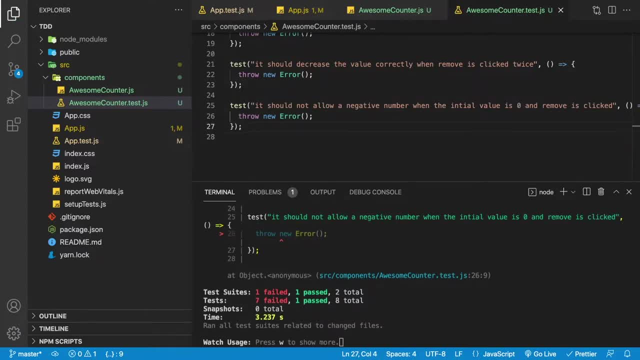 initial value is zero and remove is clicked. What's really cool about this is we have seven failing tests. Once we make all seven failing tests pass, we can then run the test and see if it's the application, and the application will work. Another novel thing about this is that we're not 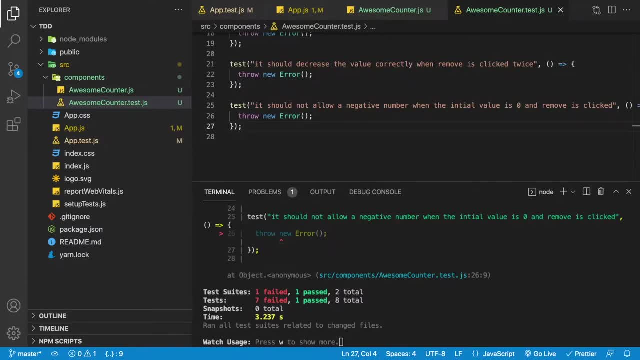 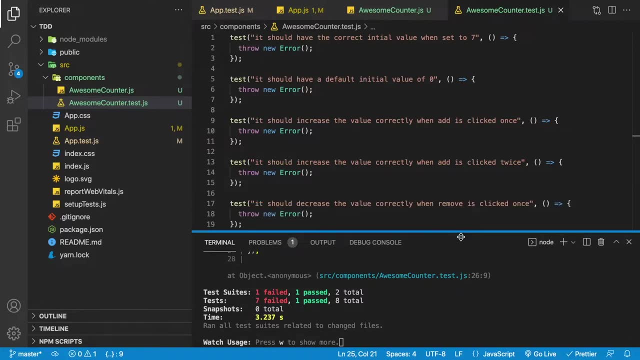 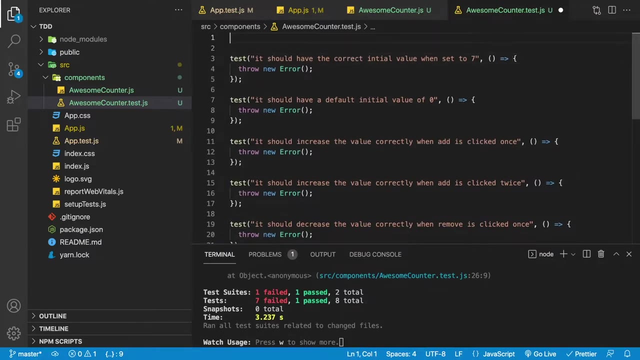 even running the application until the very end, for the simple reason that by making our test pass, the application will be fully functional. Let's go ahead and write that first test. So the first test is: it should have the correct initial value when it's set to seven. Let's go ahead and add a. 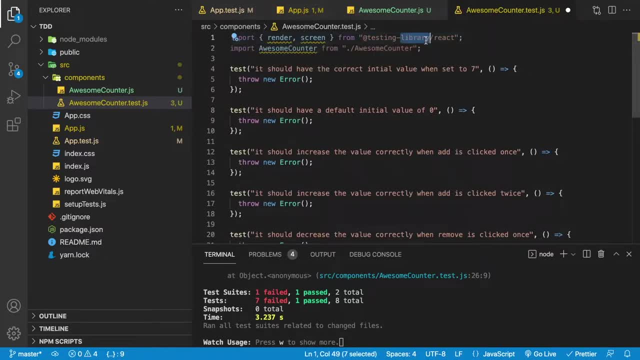 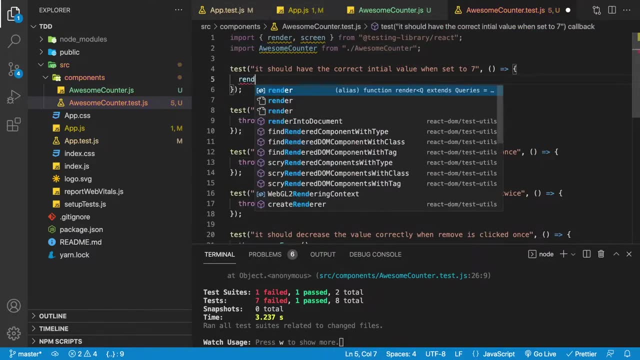 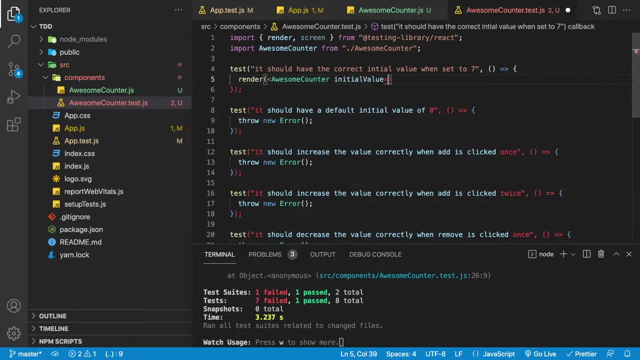 couple imports. We're going to import render and screen from testing library, And we're also going to add a counter, So let's go ahead and implement that test. The first thing we need to do is render our awesome counter. we're going to then set the initial value equal to seven. then we're going to 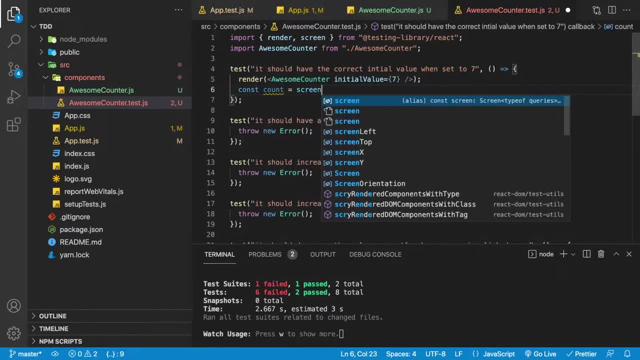 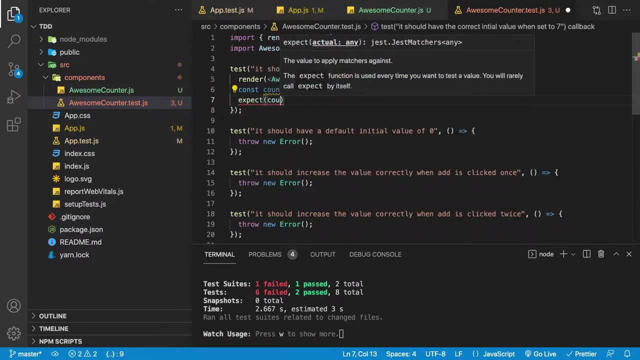 go ahead and find that count on the screen using the screen object And we're going to query by text, then what I'm going to do is I'm going to expect that count be visible on the screen, we'll save that and we'll see that we still have seven failing tests. 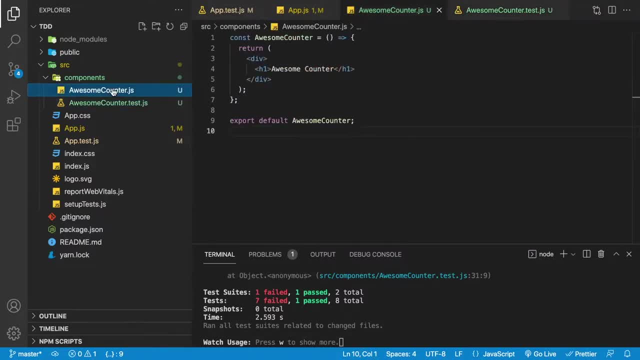 Let's go make this test pass. We'll go to our awesome counter. inside our awesome counter, we know that we have an initial value that we need to destructure. then what we're going to do is we're just going to display a span And we're going to take that initial value and display it. 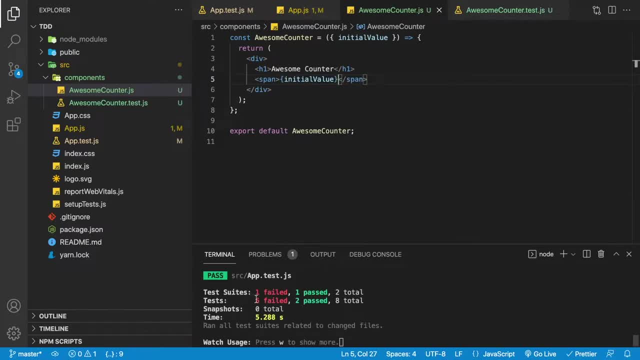 then our tests will be passing. So, as you can see, now we have six failing tests instead of seven failing tests. you're probably saying to yourself right now, Adam, why didn't you use use state? you know they're going to have to track state later. Well, I'm writing just enough. 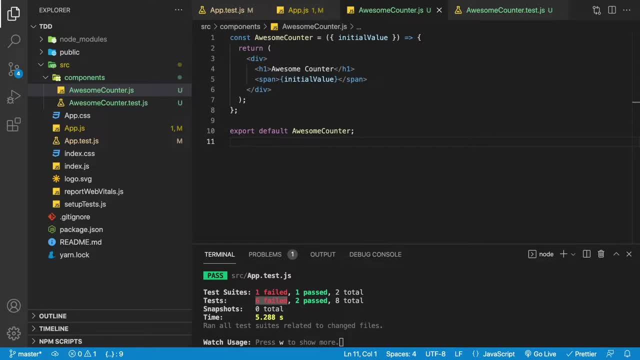 questions. So let's go ahead and run that test And we're going to go ahead and run that test code to satisfy our test. As we write each test, the functionality and the complexity inside our component will continue to increase. Let's go ahead and implement our next test. we'll go back. 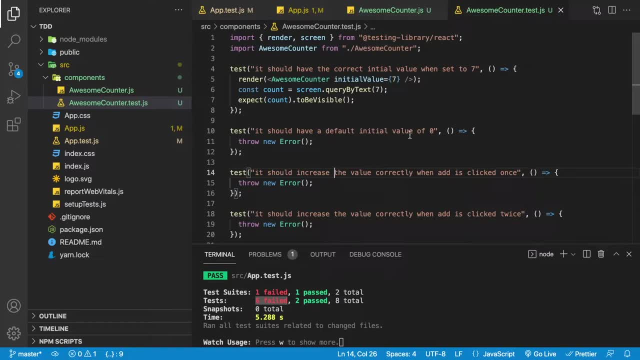 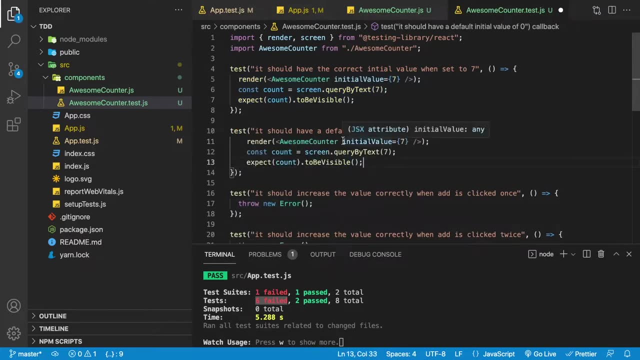 to our test over here, And our next test is it should have a default initial value of zero. What we'll do is I'm going to copy the contents of this test over here, I'm going to go ahead and remove that initial value. then we're going to look for the value of zero And we're gonna check. 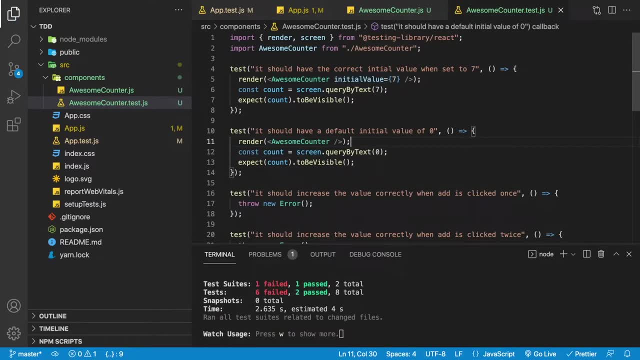 that it's a visible on the screen. go ahead and save that and we'll still have six failing tests. Well, let's take a look at that failure just a little bit closer. If we scroll up to our tests over here, we can find the test that says it should have a default initial value. 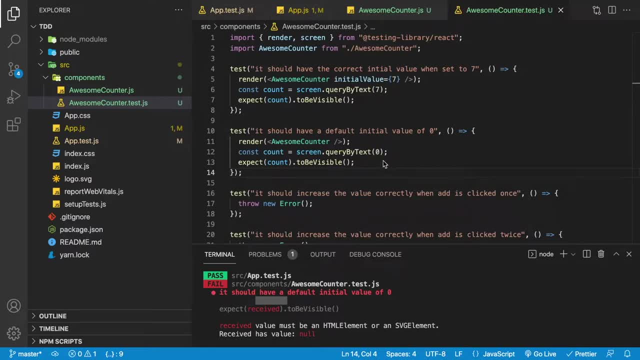 of zero. When query by text is called and it can't find a value, it returns a null. when null is returned, The expect will fail because it's expecting an HTML element or an SVG element, not the value null. Let's go ahead and make that test pass now, So we'll go to our awesome counter. 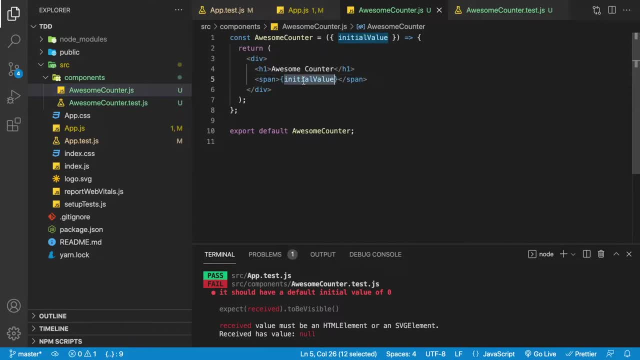 And when we get that value, all we do is display it. If there isn't a value, we want to display zero. So one way that we can do that is we can use the nullish coalescing operator. The nullish coalescing operator looks like the: 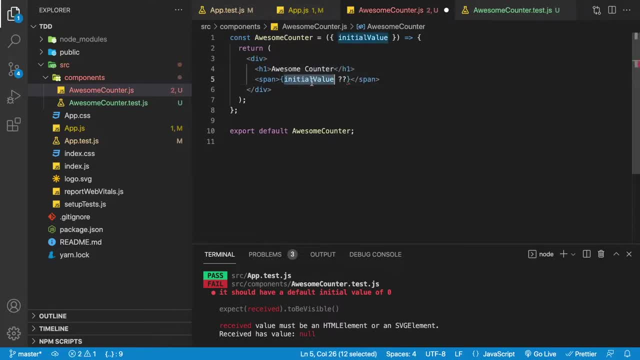 following: So you have your value And if your value is not null, it's going to display that value. But if the initial value is null, then it'll display what's on the right hand side. So if there isn't a value, we're going to say display zero. Now, if we look at our test over, 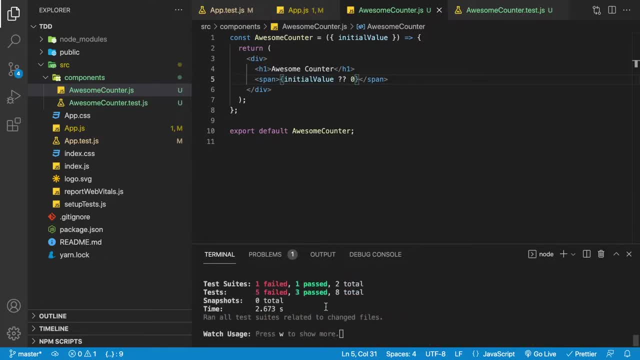 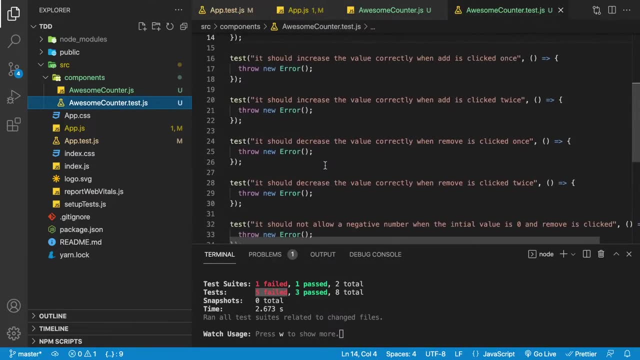 here we can see it's kind of moved on to the next test. But to really confirm that, we'll scroll to and we can see now we have five failing tests. Let's go ahead and take a look at our next test. So our next test is: it should increase the value correctly when add is clicked once. So let's go. 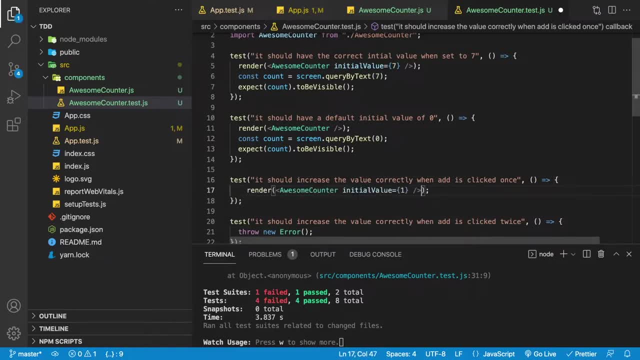 ahead and implement this test. First thing we're going to do is we're going to render that component. we'll set the initial value to one. then we're going to do is we're going to find our add button on the screen For that. we're going to go ahead and use green, get by text And we're going to look. 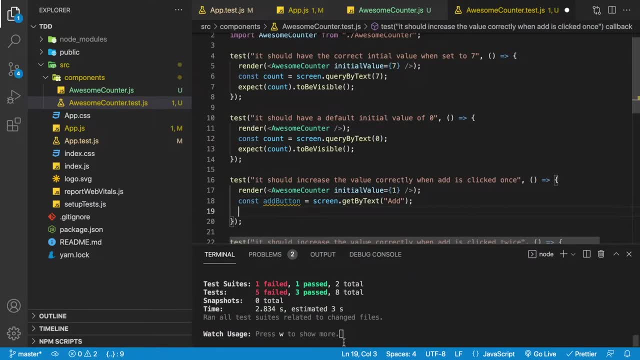 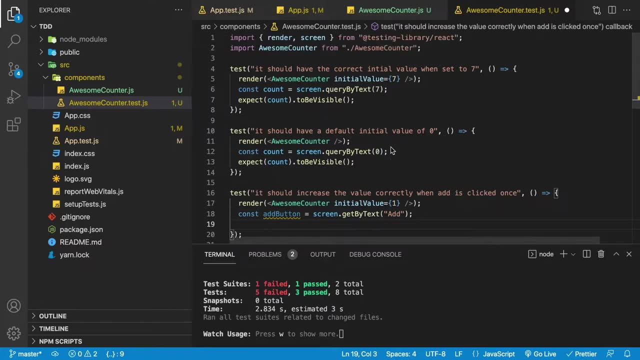 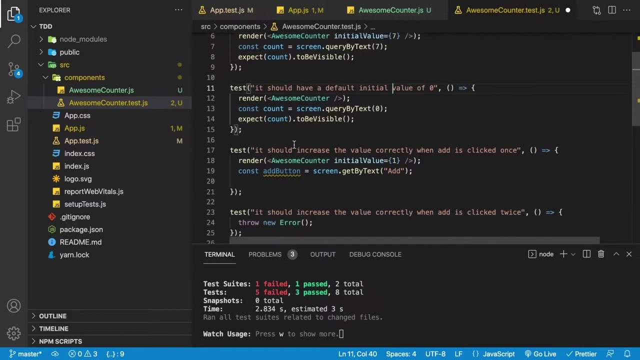 for the text ad, Then what we need to do is click the button. In order to click the button, we're going to have to go ahead and import something called user event from react testing library. So up over here we're going to go ahead and add a new import. We've added user event And then back inside our 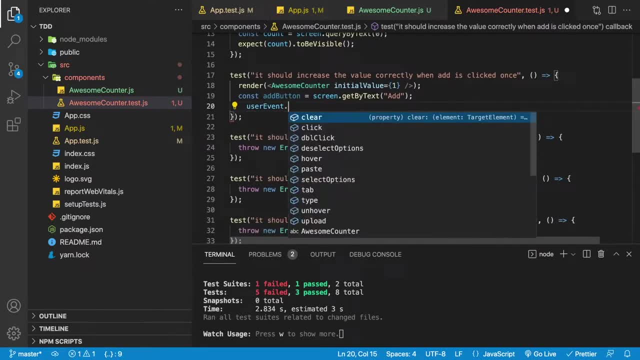 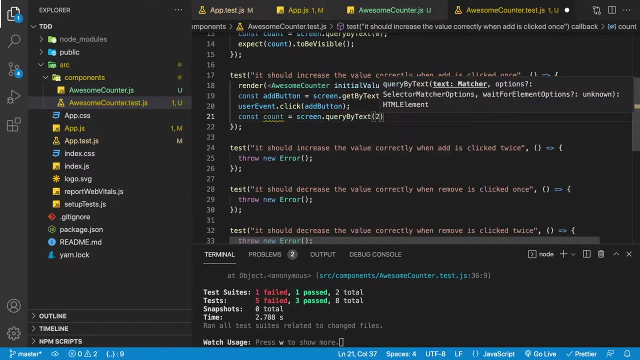 test method. let's go ahead and click that button. So we'll go user event click and pass in the add button. Then we're going to go ahead and look for the expected count value, which we're expecting to be two, And then, lastly, we'll go ahead and click the add button And then we're going to go ahead. 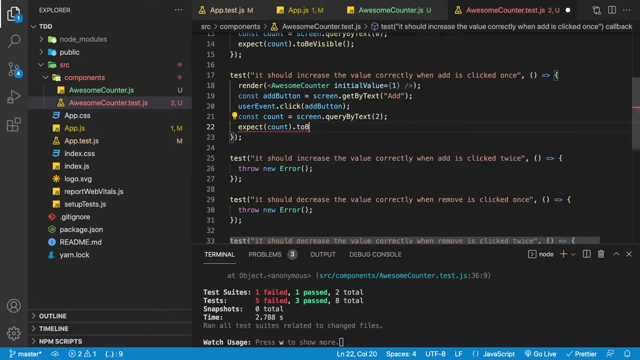 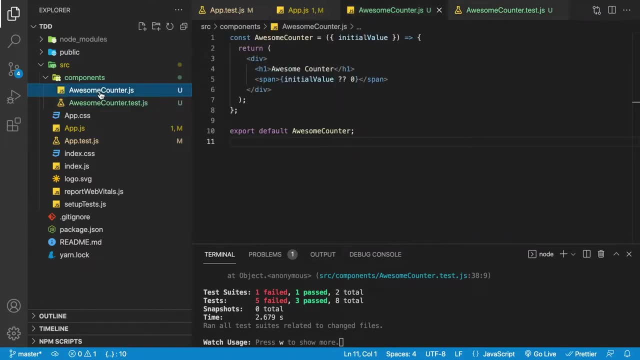 and say: we expect our count to be visible. Now let's go ahead and implement the code that will make this test pass. So we're going to go back to our awesome counter over here. Now we're going to be adding a button, and that button is going to be the add button, As you might have suspected. 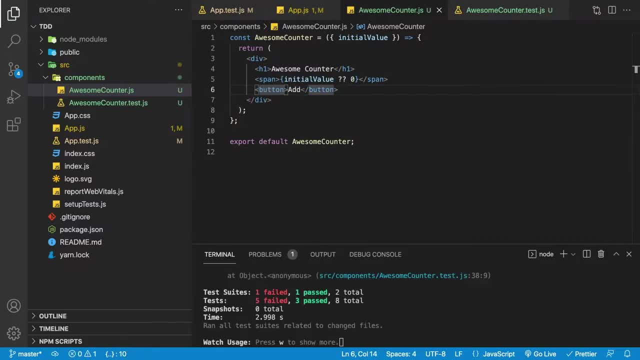 at this point we are going to need to add state In this file. we're going to be doing a big refactoring. we're going to switch from using this initial value to using the state. Whenever we do this, we're going to have a risk that we could break something, But because we have those initial 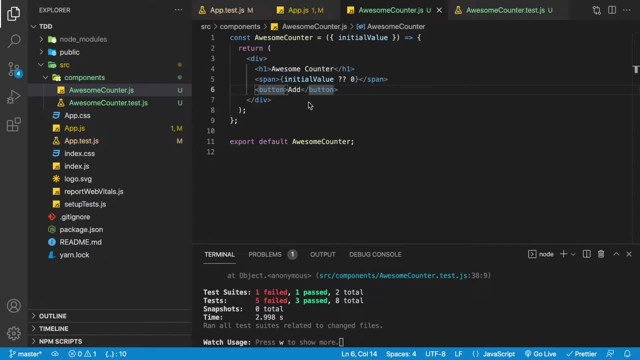 tests we wrote we can be more confident in the change that we're making To our add button. let's go ahead and add a click event So that click event we'll go ahead and execute a method called add. then we can define the add method. We'll just do that above our return and save it. 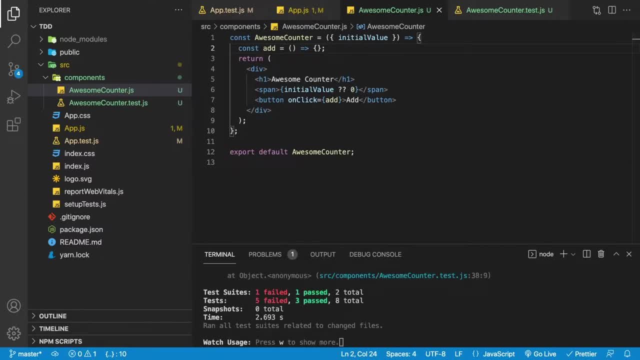 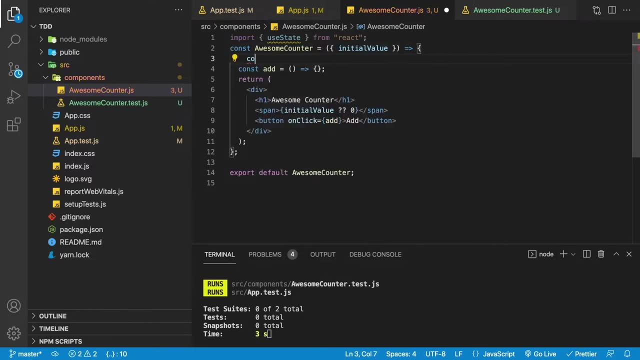 Now let's define some state for application. So what we'll do is we'll go ahead and we're just going to import view state from react. then we'll define our state. So our state will be a count And we're going to have count and set count And we're going to make 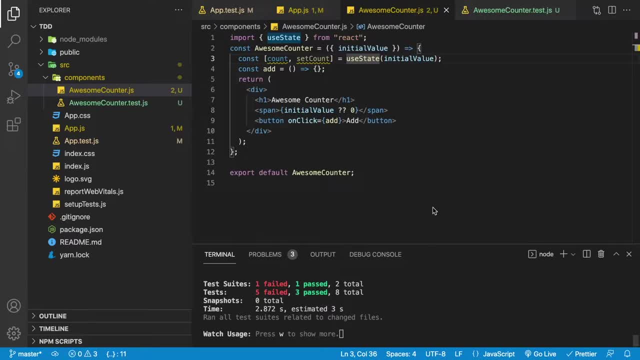 that equal to use state and pass in the initial value. Then below over here in our span we'll go ahead and we'll start using that count of value. Now what you'll notice over here is we're getting one extra failure. So if we look at our test over here we can see it should have a default initial. 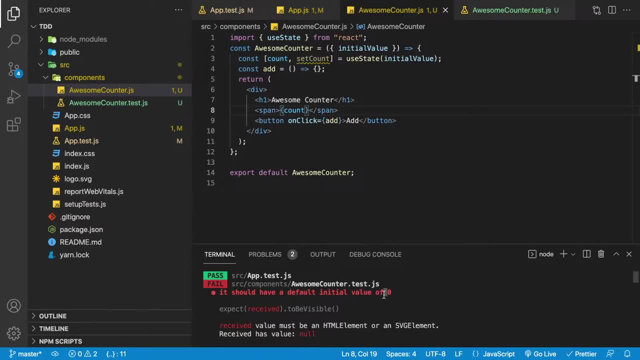 value of zero. that test was passing before, But with our new refactoring it's now failing. So the way that we could fix this is, when we set our initial value in the use state, we can use that same knowledge coalescing operator, And if there's no value, 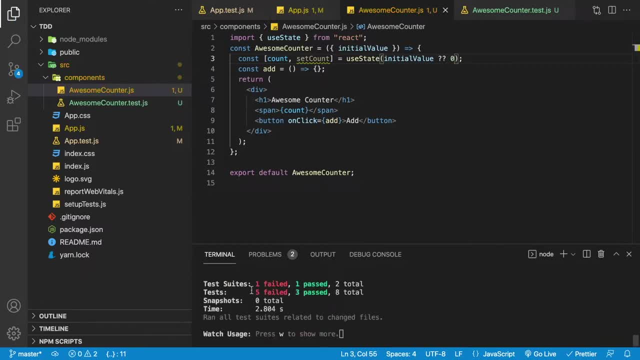 then use the value zero. Now the number of failures is back to five. What's awesome about these tests over here is that when we did this refactoring, we actually removed a piece of functionality. Without these tests, we might not have remembered to add that functionality back. 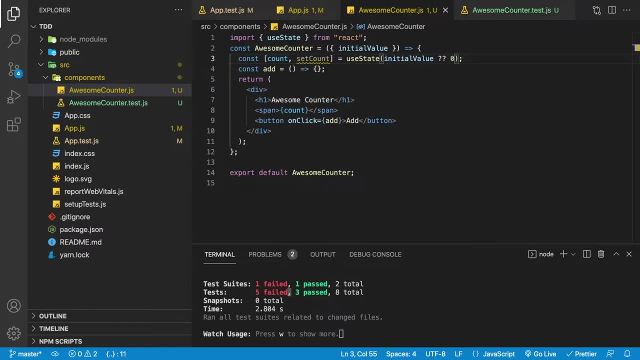 So these tasks gave us a safety net in which to work. Now you won't run into that situation where you have to deploy your code into production and find out that you have a bug. At the end of the day, testing will help you keep your quality really high. Let's go ahead and implement the add method. 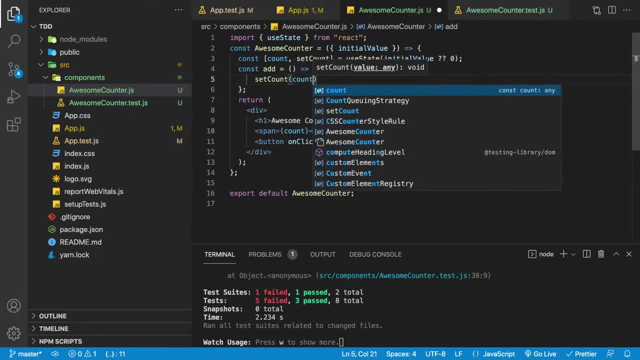 over here. So we're going to call our set count. Now we could call set count with count plus one, like that, which will work Well. so we'll run that and we'll see that we have four failing tests now. But, alternatively, a better way of doing this typically is to use a function. So this way, 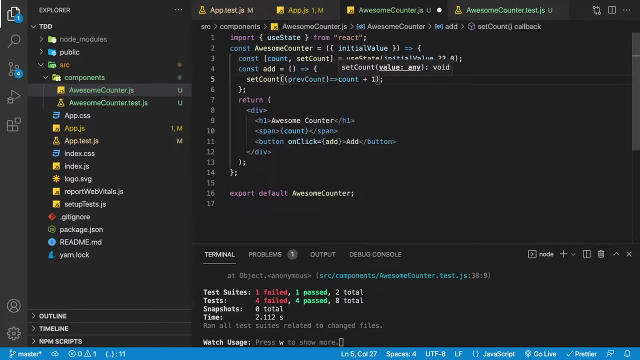 if you call these really quickly in succession, you might get an incorrect value, But this will always make sure that they're called one after another for every set count that you've called or every state change that you've done. we're going to do over here. we'll pass in a lambda function with the previous count and go. 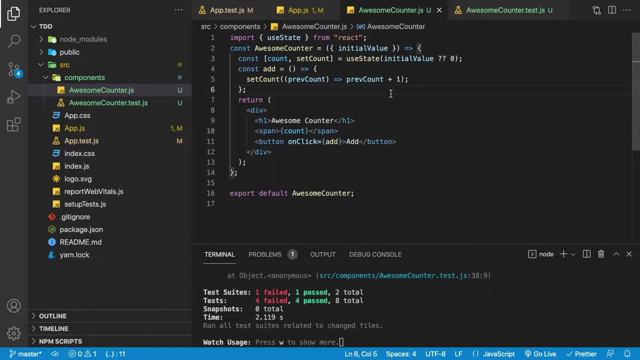 previous count plus one. we'll save that And because we have these tests once again, we have that confidence And you can see that we only have four failing tests instead of the five that we had before. Let's go ahead and write our next test, So we'll jump back into our awesome counter test. 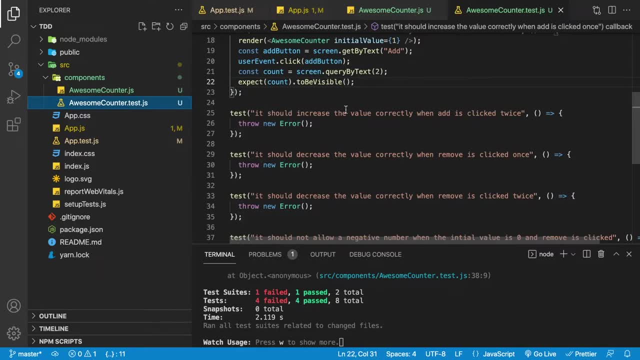 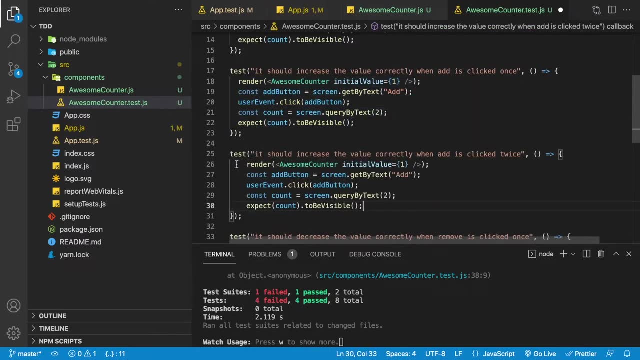 JS And looking at this one, our next test is it should increase the value correctly when add is clicked twice. So what I'm gonna do is I'm going to copy this method over here And then for this method over here. what we're going to do is we're going to expect that when add is clicked twice over here. 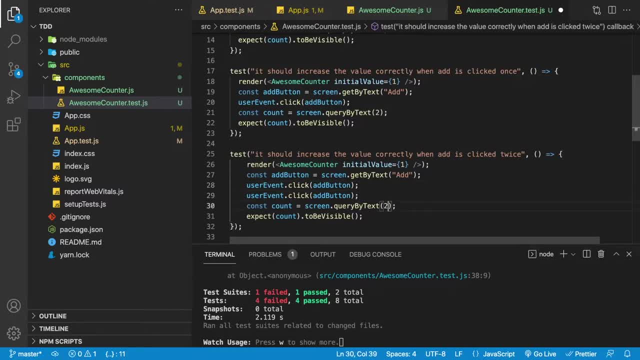 so we're going to user event dot. click Add button two times. then we're going to expect our result to be three. will run this test and it will pass. we don't have to go update any code because it's already passing over here. Let's go implement our next set of tests. So now we're going to. 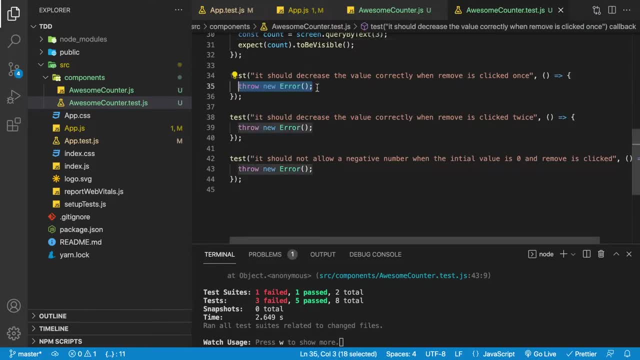 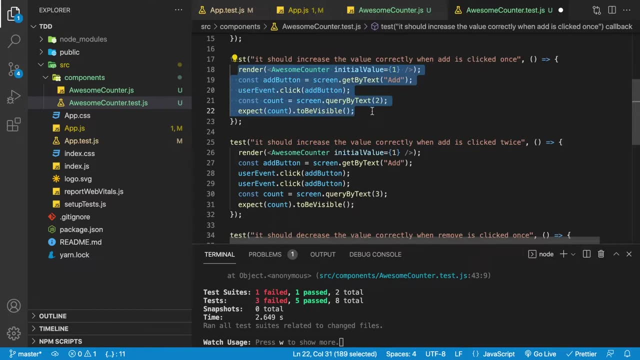 implement the remove button. So let's start by writing that test, This test, over here. it's going to be very similar to our ad, So we're going to go ahead and copy our ad test, the first one, where we only click once. we'll paste that in over here. then we'll just 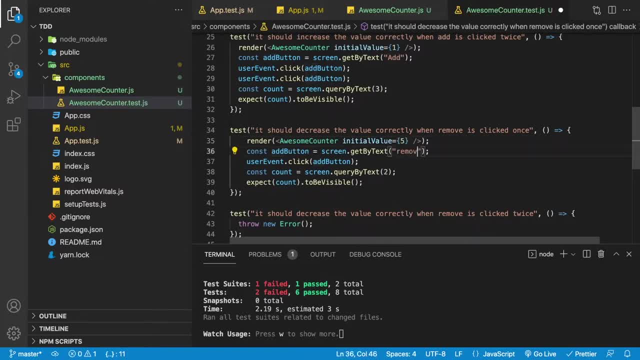 modify our tests or initial value, we'll set that to five. we're going to look for the text that says remove And we'll rename our button there from add button to remove button And then, lastly, because we're clicking the remove button once, we expect that value to be four. While we're here, 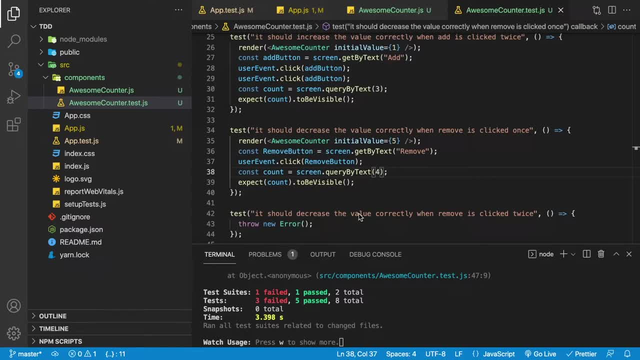 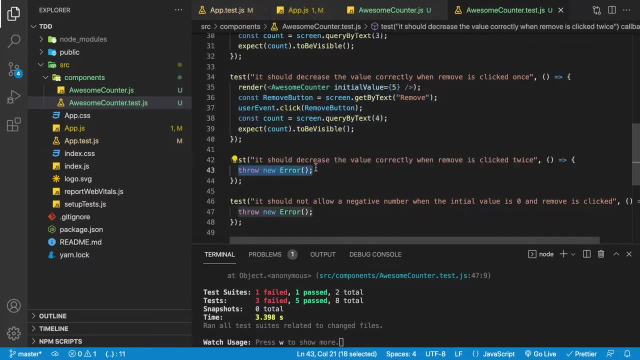 we might as well implement the next test So it should decrease the value correctly when remove is clicked twice. we'll go ahead and just copy the test that we just wrote, And what we're going to do is we're just going to modify it, So 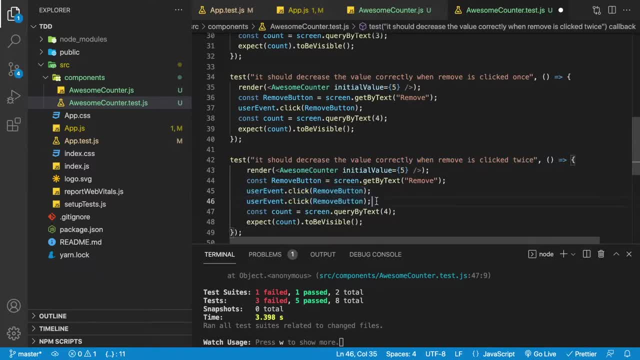 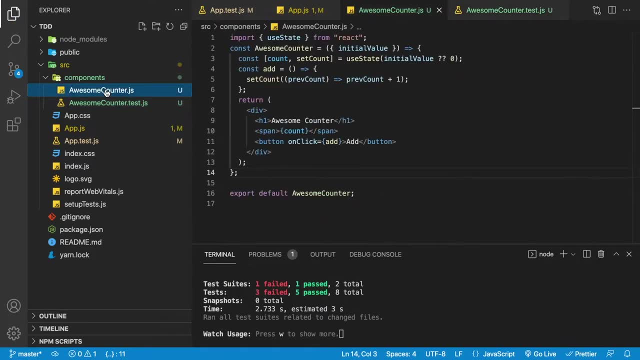 we're clicking that button two times over here, then instead of the value being equal to four, the value should be equal to three. Now we can go back to our awesome counter and implement our remove button. So I'm going to go ahead and just like our add button over here. I'm going to copy: 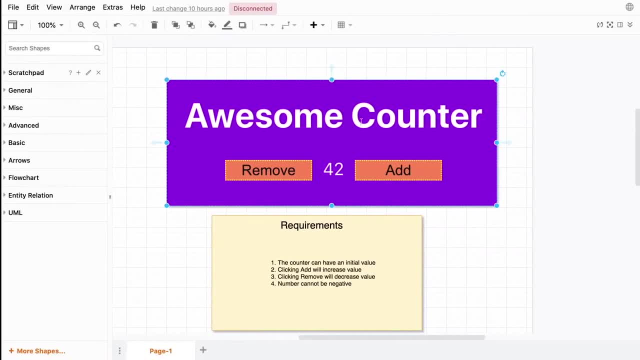 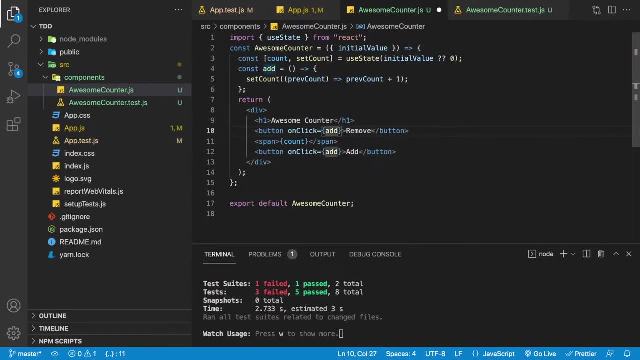 that I'm going to put that before the span, just like our mockup. we have the remove button on the other side of the text, then I'll just update this text over here So it says remove. we're going to have a new function that we're going to add, called remove. 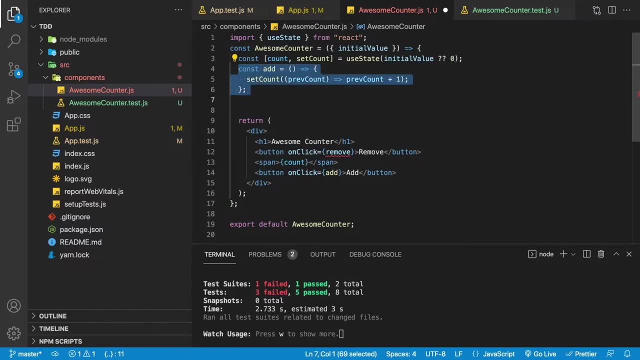 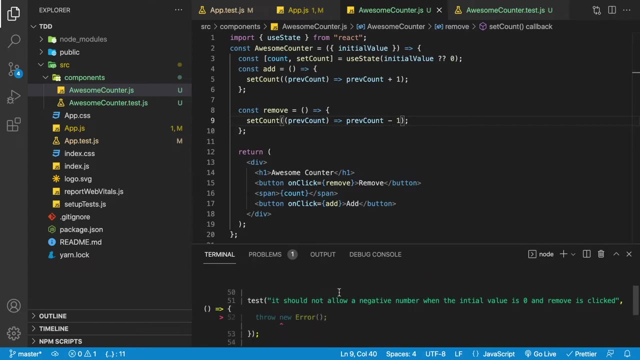 we can go ahead and add that function, And you know what? I'm just going to copy that add function, rename it to remove, And then the only modification I need to do is, instead of adding will be minusing. And now, if we save, we're going to get our test passing, But now we're just down to one failing. 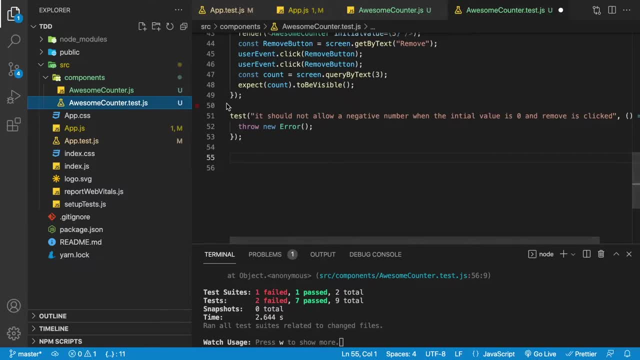 test. So let's go ahead And implement our final set of tests. So the test we have right now is: it should not allow a negative number when the initial value is zero and remove is clicked. In addition to that, let's go ahead and add one more test that we could implement. we're going to do is we're going to say. 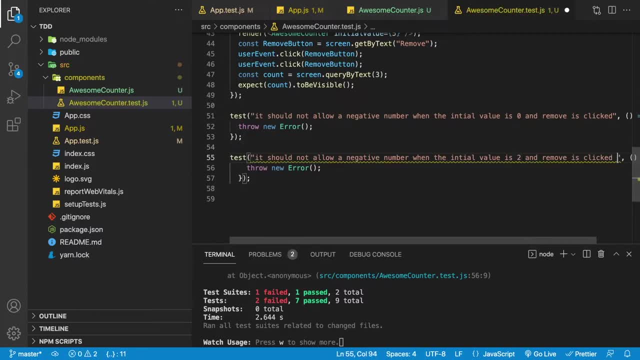 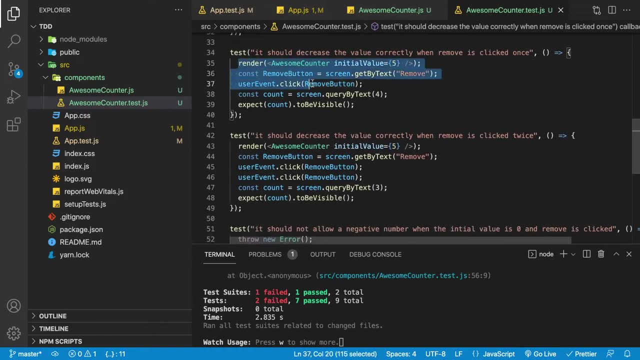 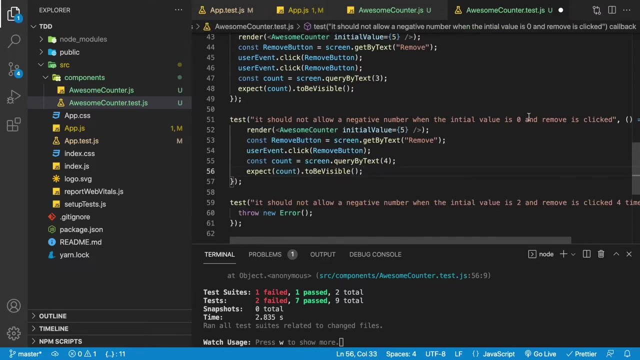 when the initial value is two and remove is clicked four times. this test is very similar to the test we wrote above for removing. So what to do is we go ahead and copy this test over here where we clicked once. I'm going to paste that in over here And we'll make modifications. 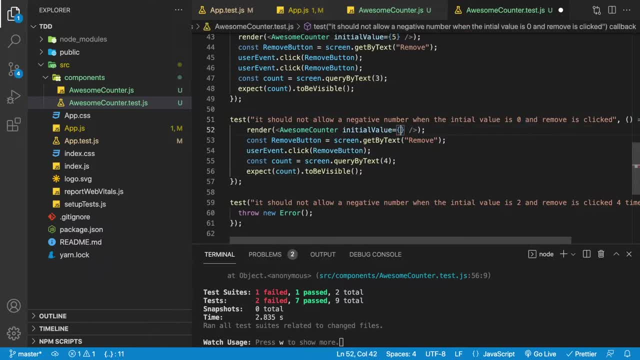 based on what the test tells us. So the initial value will be zero. I can omit initial value and it'll be zero, or I can put zero in. then we're only going to click Remove once And we're expecting the value to still be zero. Let's run our test And we still have two failing tests. Then let's. 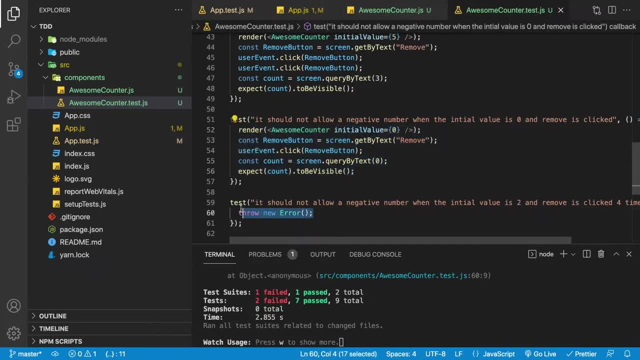 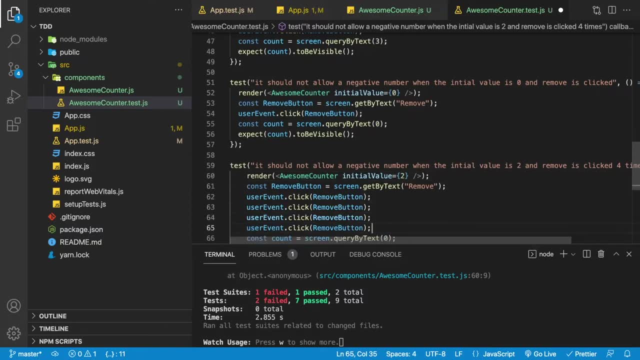 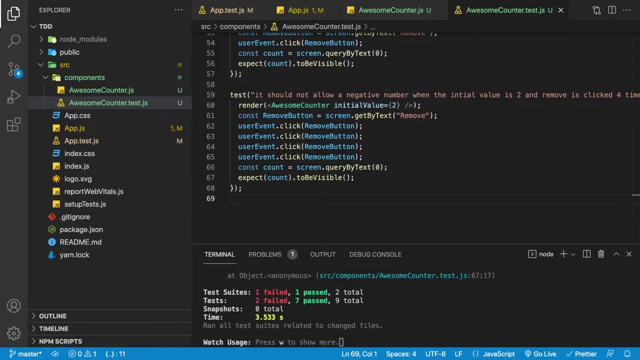 go ahead and copy this once again, paste it in over here. Now our starting value for this test is going to be two, And then we're going to click Remove four times. So there's my four times I click Remove, then our value should still be zero. If we take a look at: 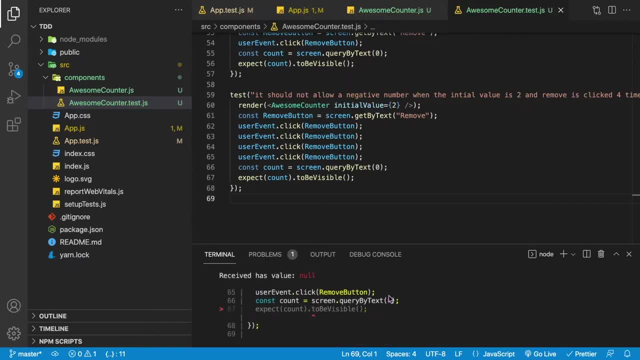 our tests. we can go ahead and see that the failure is occurring because it's unable to find that zero text on the screen. And the same thing for this test as well. you make this pass. we're going to go inside our awesome counter, inside our awesome counter, inside the remove. 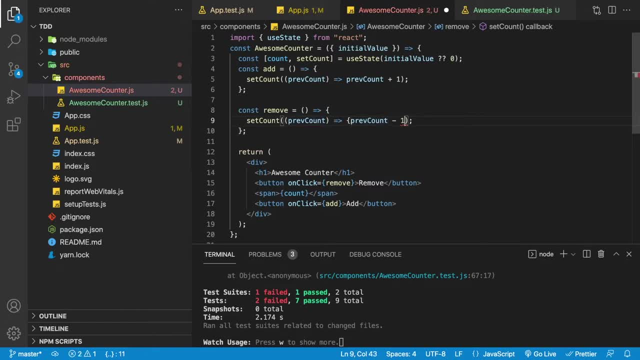 function. we're going to modify this method over here So we can have multiple lines instead of just a single line. what we're going to do is we're going to take the value of previous minus one and store that in a variable. then we will check our result and see if that's less than. 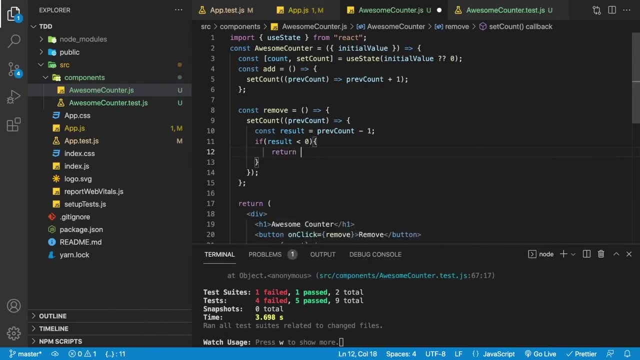 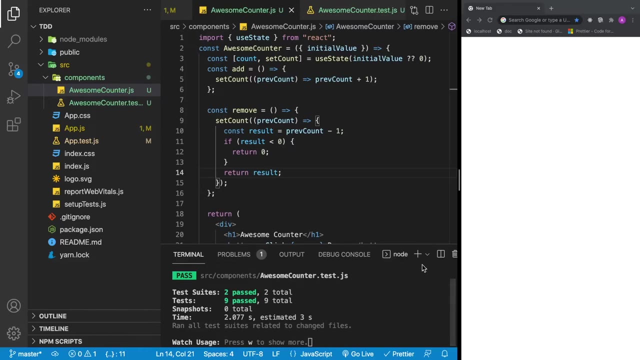 zero. If it is less than zero, we are going to return zero. Otherwise, we're going to return the result. All right, there you go. Now we have all the tests passing for application. This means that when we run our application, we'll see it working. We'll go ahead and run our application. 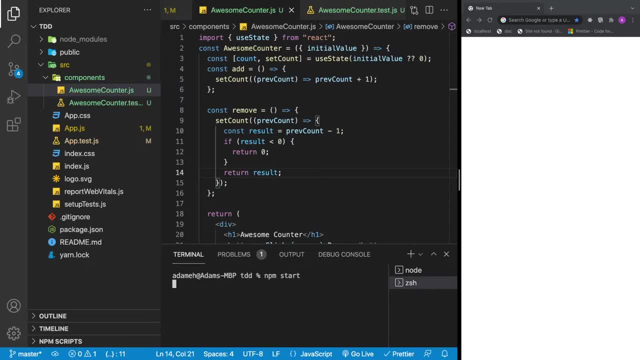 So just open up a new terminal there And I'll do npm start And there you go. we have our application. So let's give it a test run here. It doesn't doesn't look very nice yet, So apply a little bit of styling shortly, But first let's give these: 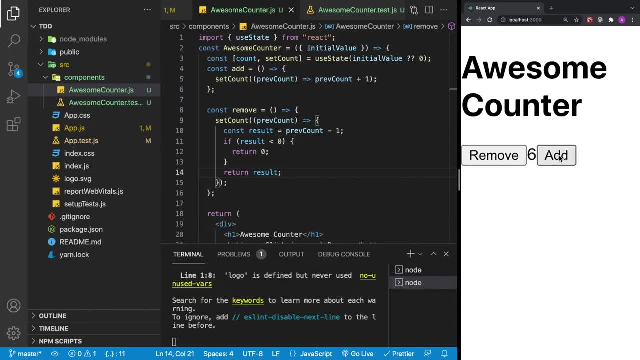 buttons a try. If I click Add, we can see that value increases. I go ahead and click remove, we can see that value goes down. And also our negative check is working to. every time I click remove, I can't go past zero into a negative number. This is perfect. We wrote that entire. 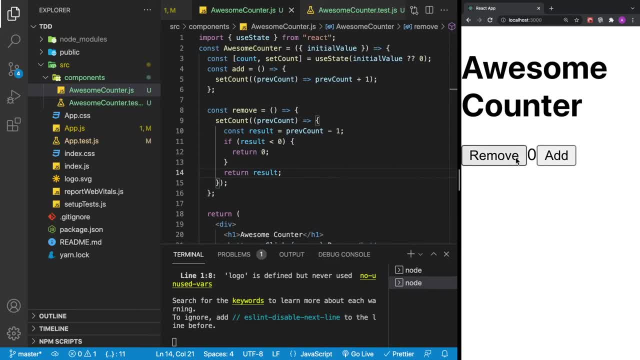 thing with tests. we never ran the application once, And once we got to the end over here, we ran it and everything worked because all our tests were passing. Let's just do one last thing for this application. Let's go ahead and make it look nice. We're going to go to our indexcss And 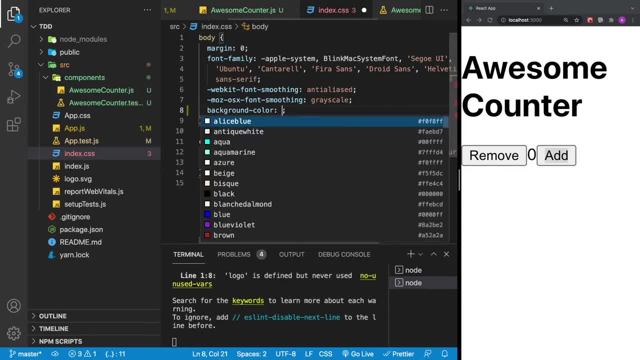 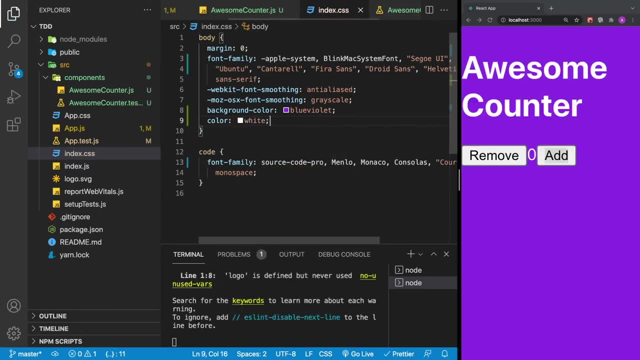 we're going to apply a few properties to the body. we're gonna go ahead and apply a background color. I'm going to apply blue violet. then we'll also set the color of the text to white and save that. You can see that looks a little bit more like the mockup. Then we'll just apply a few styles. 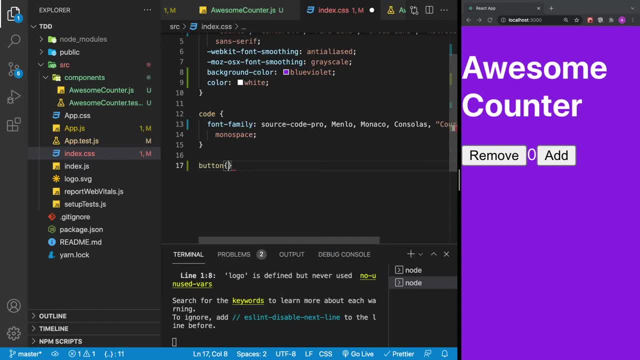 to our buttons, So I'm going to add our button over here. We're going to give them both the same width of 80 pixels, we'll give them a margin left and a margin right of 10 pixels, a background color of coral, And we're going to go ahead and apply. 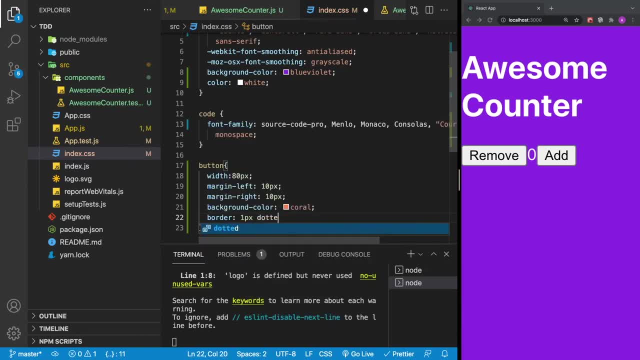 a border to them as well. We'll make it one pixel, we're going to use a dotted yellow And, lastly, the color of the text will be the color black. go ahead and save that. And now, if we just expand our